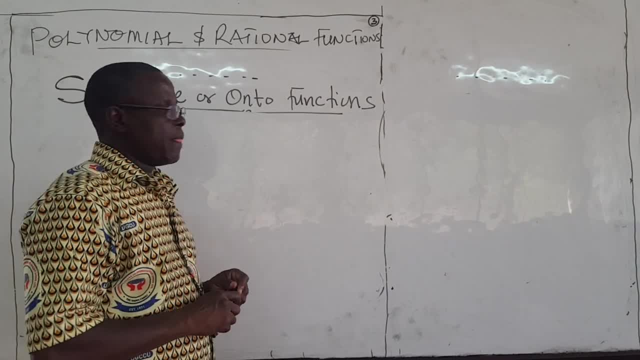 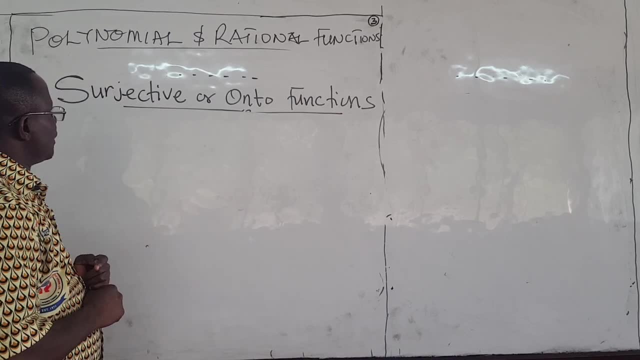 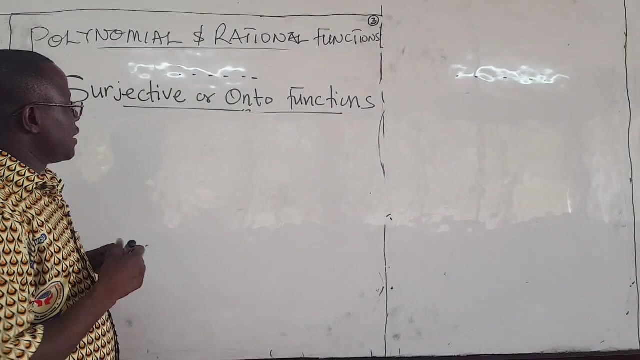 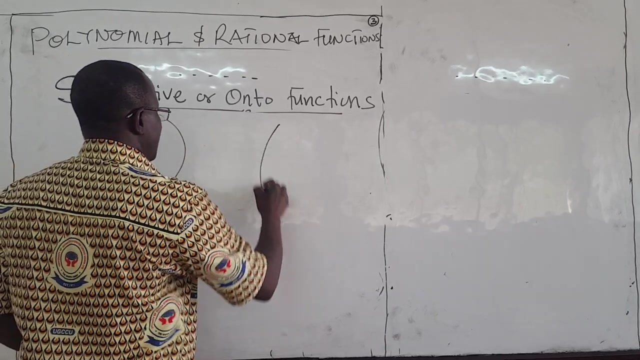 Hello guys, you are welcome back In this lesson. we want to study subjective or onto functions. In other words, when we say that a function is onto or subjective, that is all we want to look at. We obviously start with this: a function marking an element from 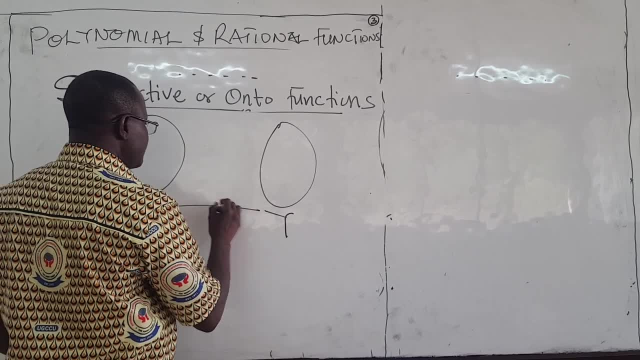 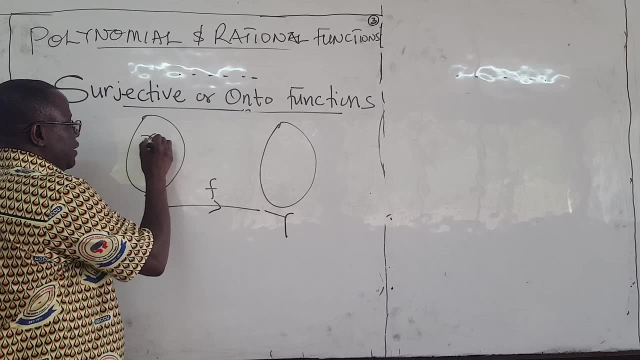 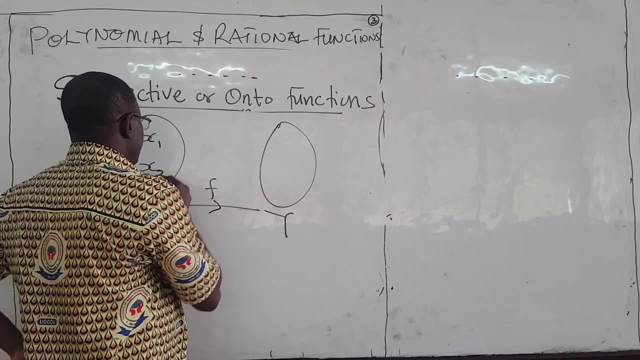 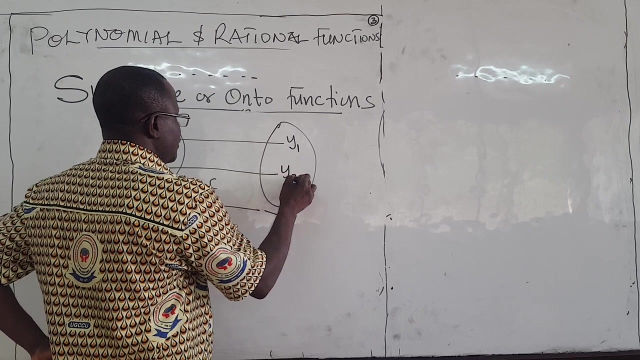 x to y, I'll call it f. Alright, so you have elements in here. Let's say you have x1,, you have x2, as we've done before, and then mark two elements corresponding elements here. So let's say this guy marks to an element y1, this marks to an element y2.. 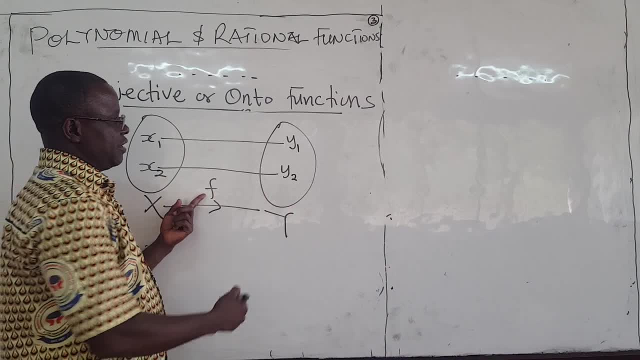 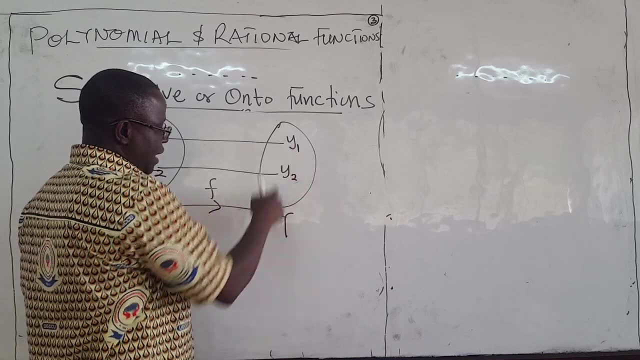 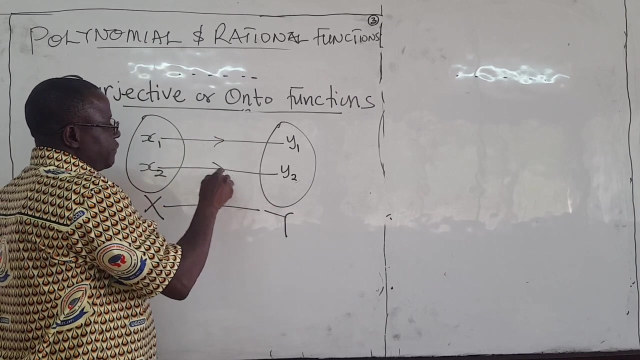 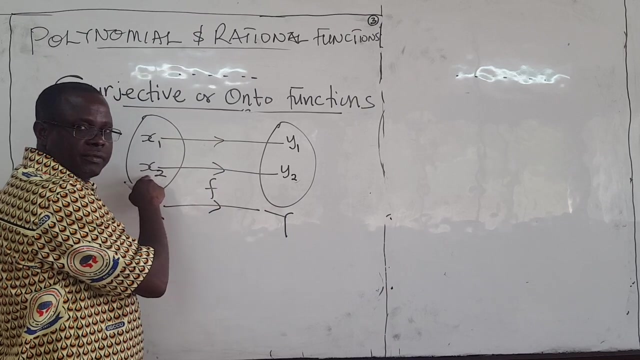 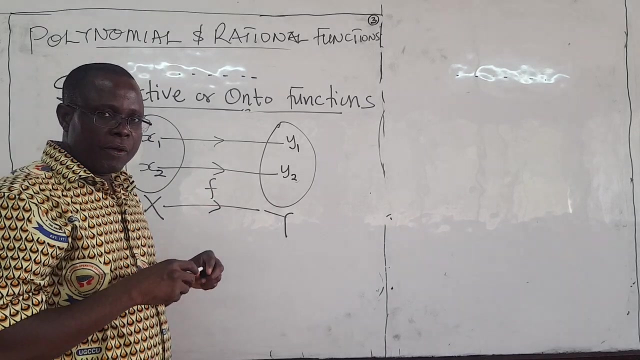 We have already learned that the range of f is this: functional values. Alright, the subset of functional values of f that are in here, y form the range. Right Now, if for every element here in the code domain, for every element here, I can find the corresponding x in x in the domain of f, then the function f is set to be onto Okay. So suppose that. 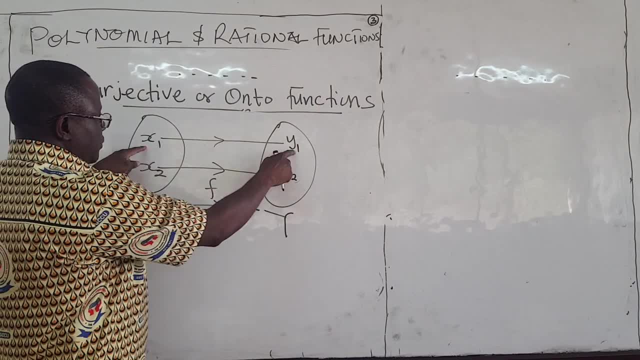 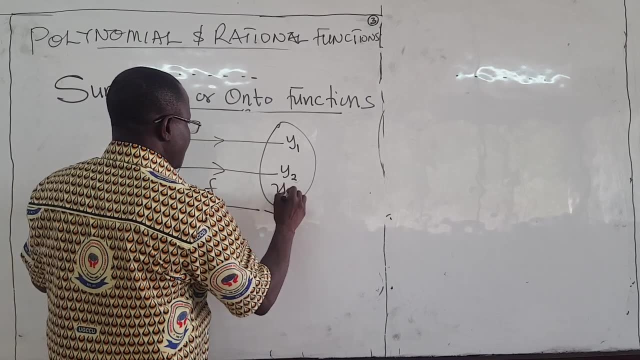 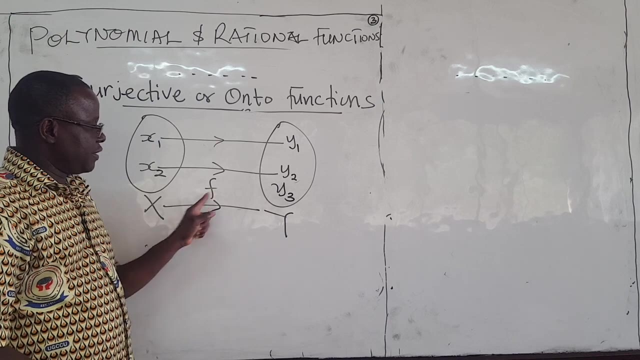 I have the same thing: x1 marks to y1,, x2 marks to y2.. Suppose that I have an element here- let's call it y3, and y3 doesn't mark to anything here. okay, Then this function will not to be onto, or? 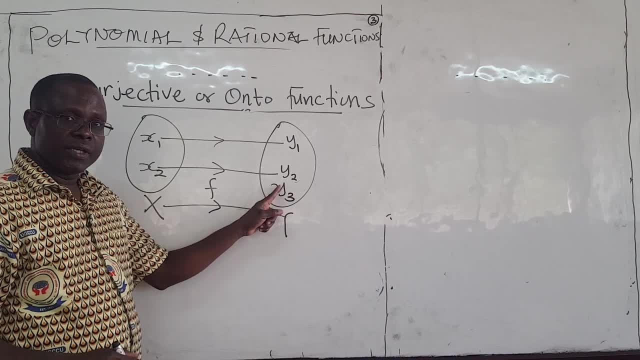 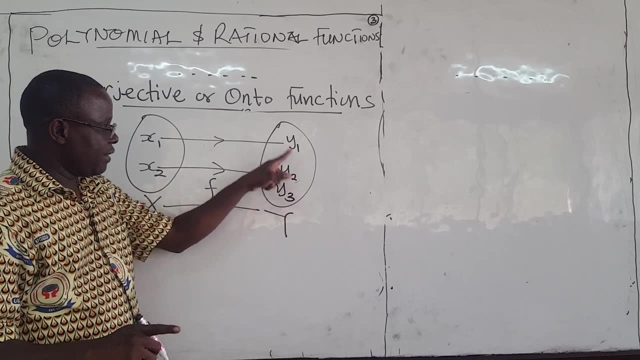 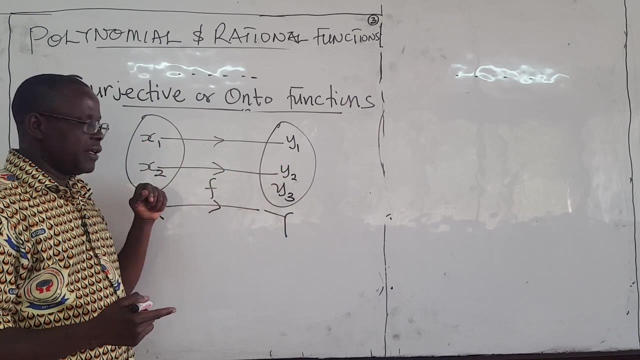 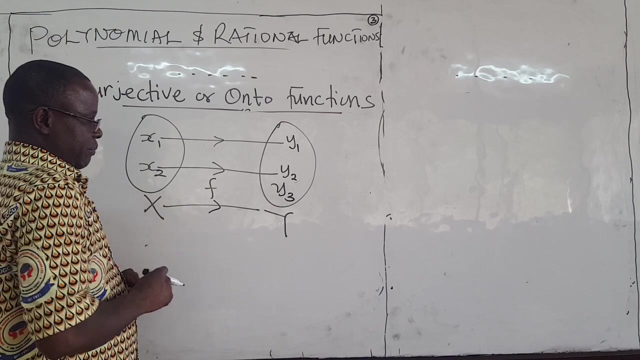 subjective, because I can find an element which is this for which there is no corresponding x here. so if you can find an element y here such that there is no corresponding element here in x, then you see that f is not, uh, subjective or onto. okay, so that is. that is really the um, the basic. 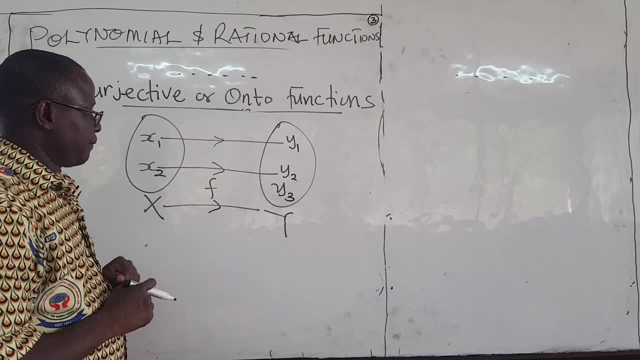 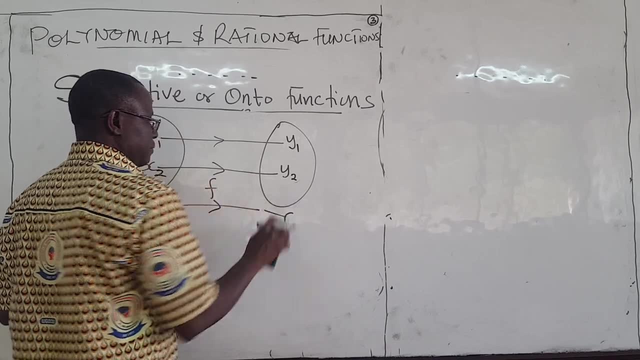 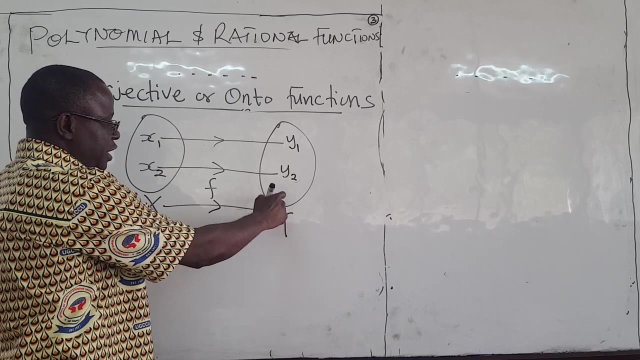 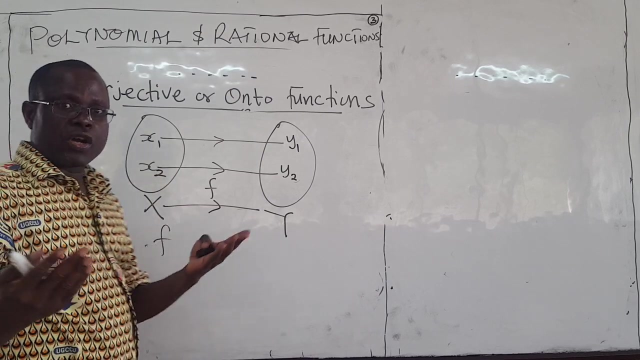 idea of what an onto and subjective functions are. okay, uh, which means that for uh onto functions, functions that are onto, the range must be equal to the codomain. otherwise, if I pick any element here in y, I must find the corresponding element here, so often times, if you are not sure, oftentimes 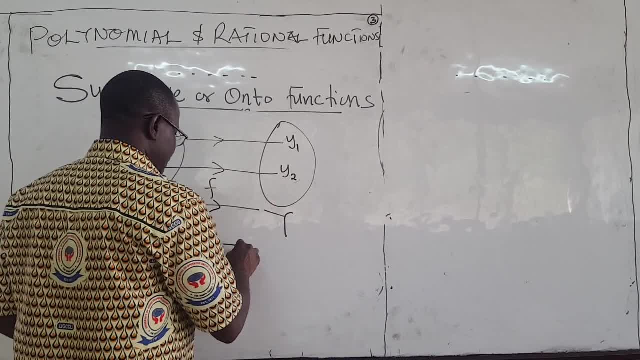 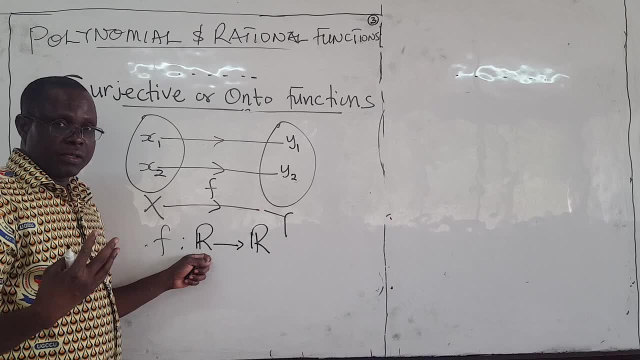 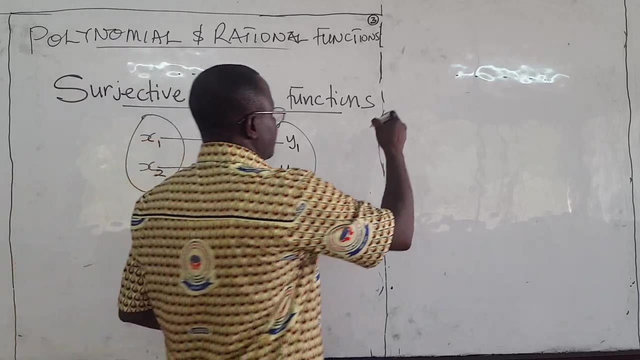 assume that f is moving from the space of real numbers to the space of real numbers, so this y will be the set of all real numbers, and actually the set of all real numbers. all right, good, so let's use an example to illustrate this. so the example. 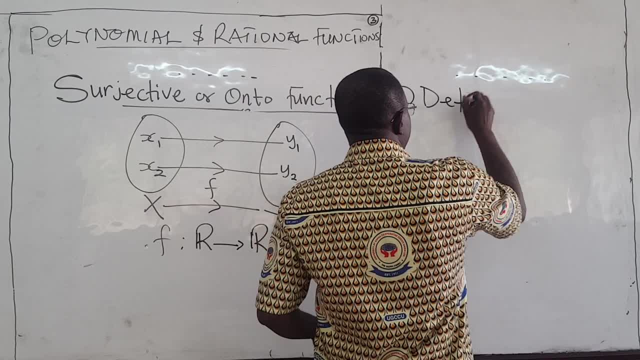 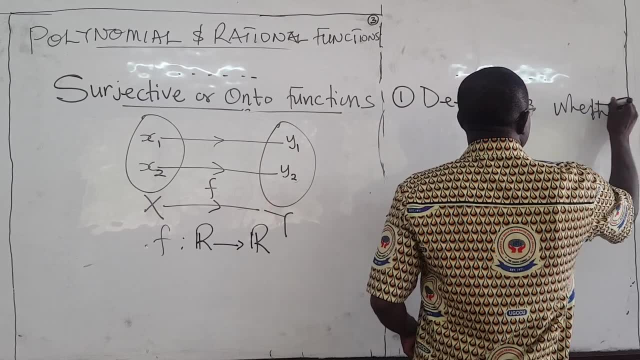 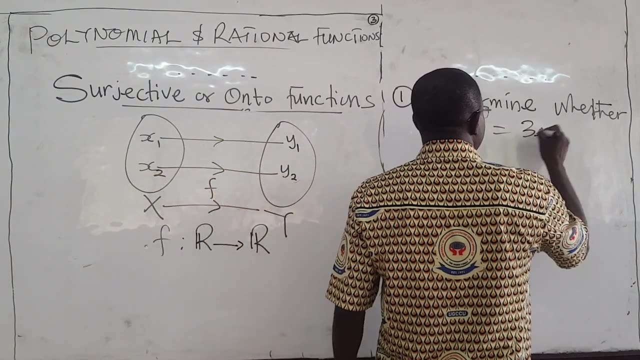 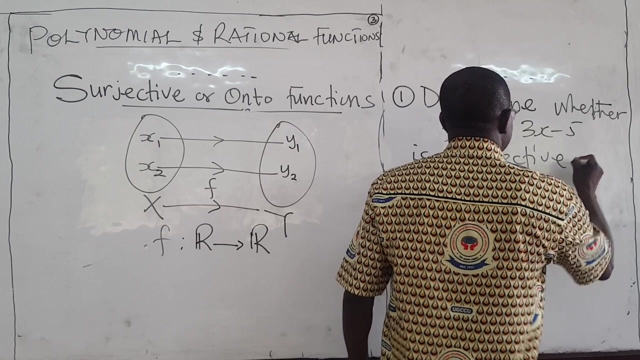 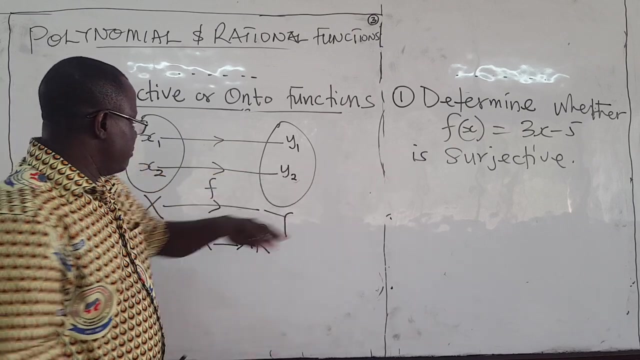 let's determine. we want to determine, determine whether, whether the function is- uh, let's leave something up- same function, f of x is equal to 3x minus 5, is subjective? okay, subjective, or onto the same thing? all right, all right. so so, again, before we do that, 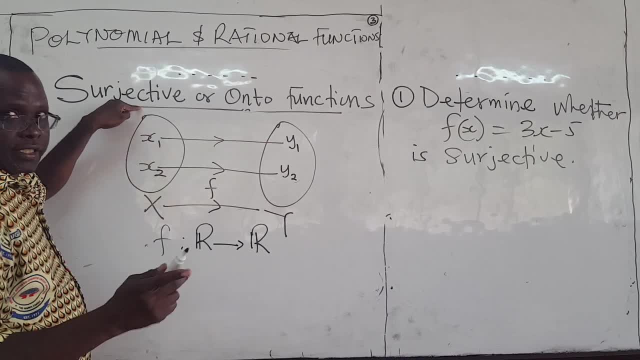 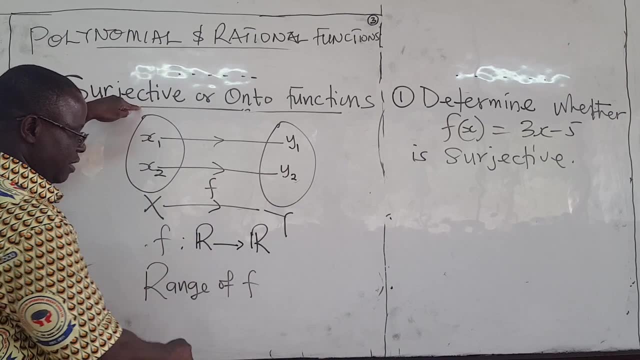 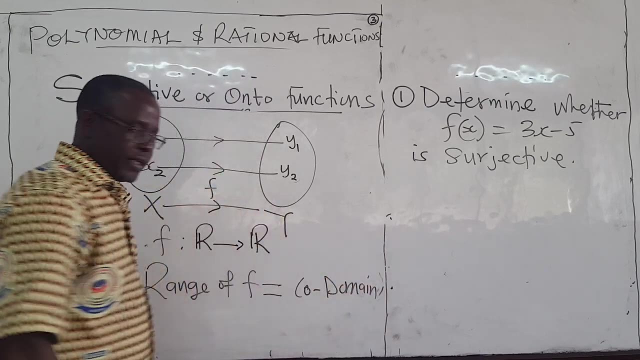 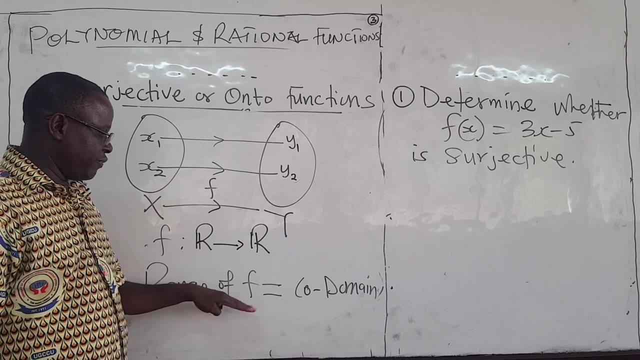 i'm saying that the function is onto or subjective. okay, then the range, the range of f of the function must be equal to the co-domain. this is important, all right. so if the co-domain is the set of all real numbers, i expect that the range of f will be the set of all real numbers. 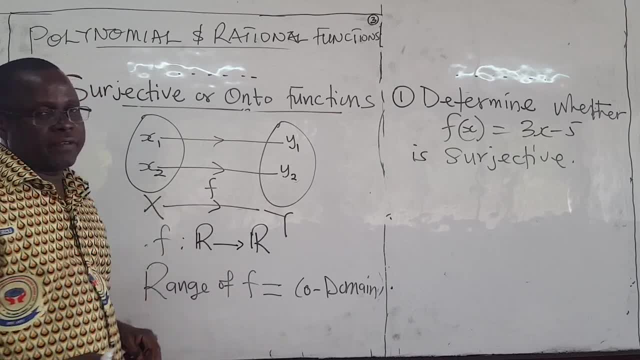 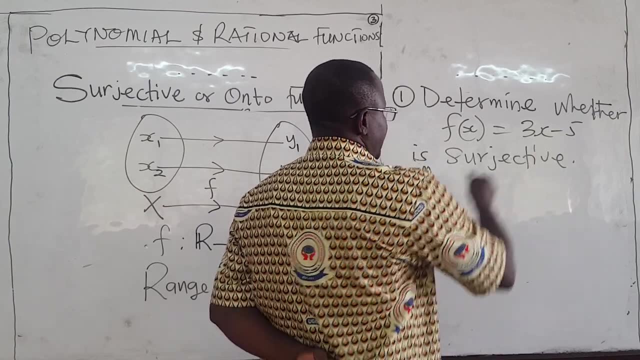 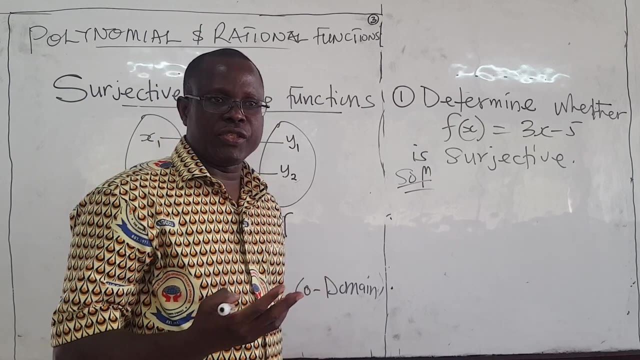 if that is the case, then, um, you can say that the function is: uh is onto, all right. so, let's, let's reach over this. so let's reach over this f of x. okay, i want to use different fields in function in every j. so we do if f of x goes together. 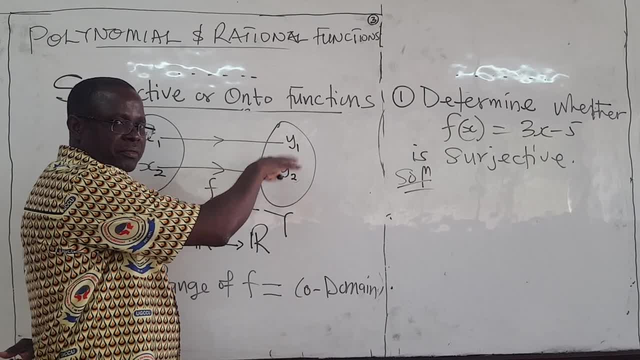 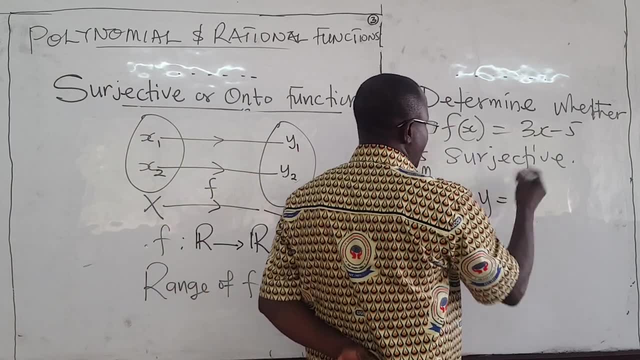 we're looking at the function f of x right once for every t. there is no function of x in t. under the code that part is the function of x, classic function. when you complete this, you will solve for x equal to 1, x minus 5, x, e to f of x. right, we want to determine whether it is onto or not. well, so the idea is very similar to what we did. we are trying to find the range of functions right. you can imagine that for onto functions you're concerned about the range right in the code doing okay, so the idea is very similar. so what you do is that your late what we call x from the transform and 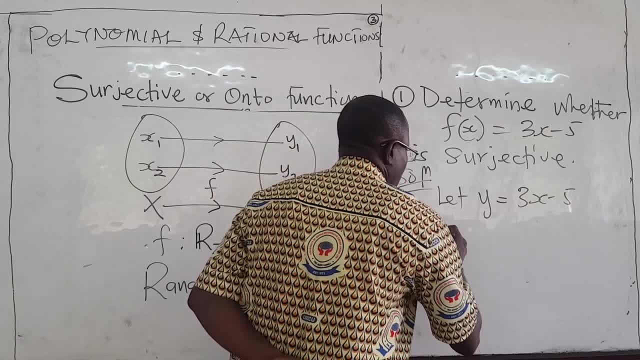 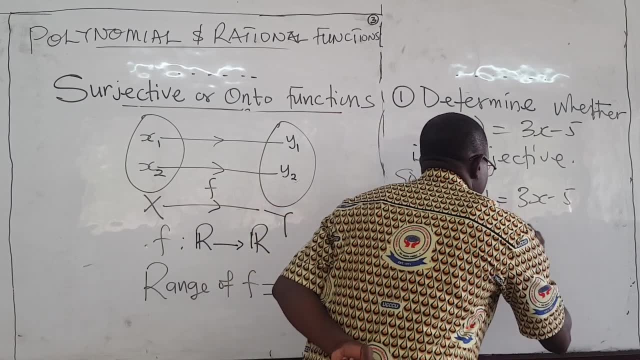 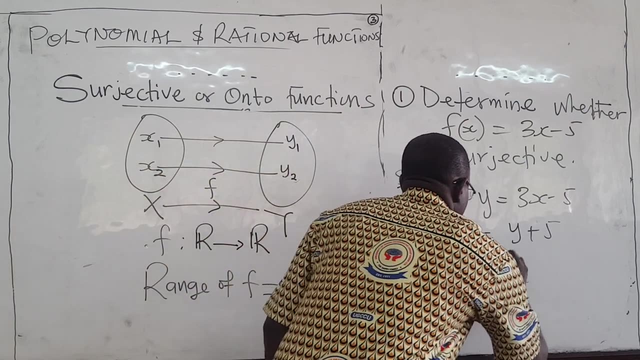 and then you solve for x in terms of y. So um break x to be y plus 5.. So, like 3x will be y plus 5, I'm solving for x. divide 2 by 3, x will be equal to y plus 5, all about. 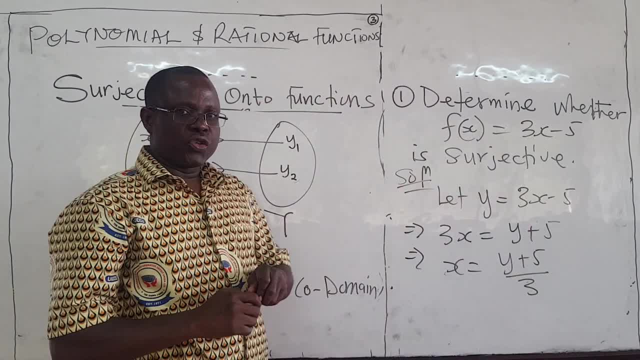 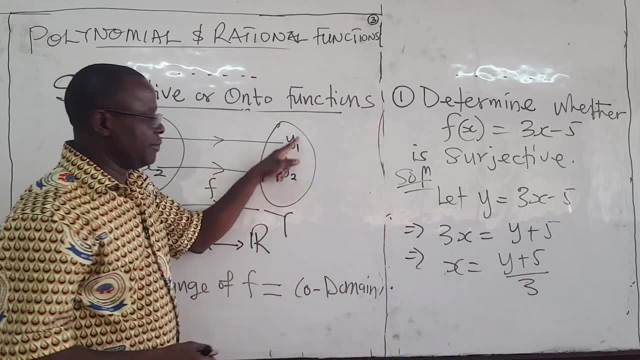 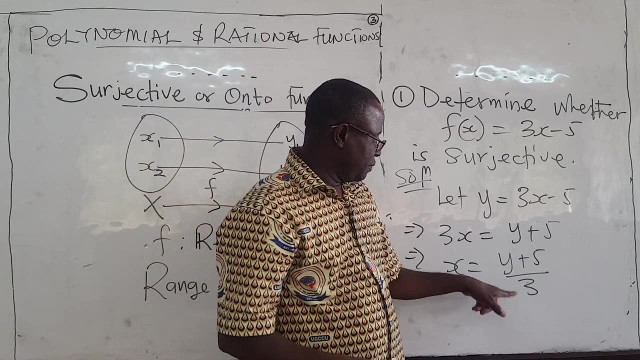 3. Okay, Good, And so once we get here then ask the question: If I pick any word, remember- if I pick any y, will I get a corresponding x? In this case, it's true, I can pick a positive. 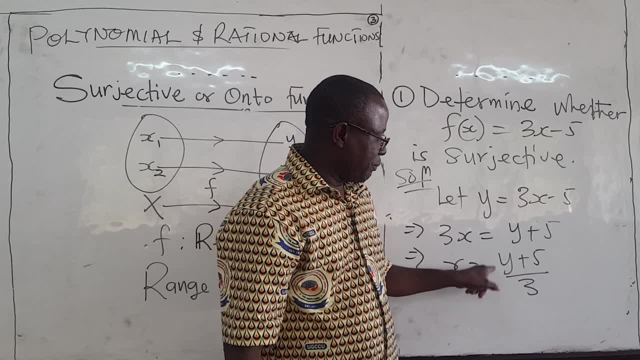 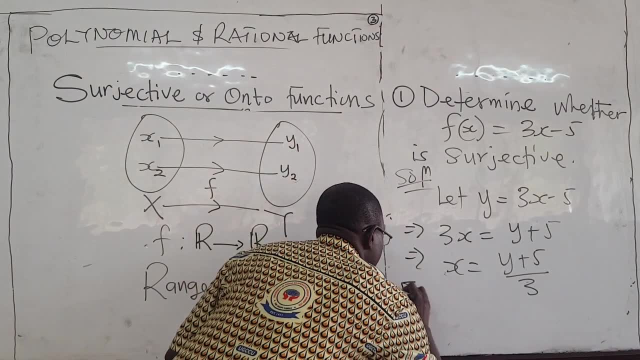 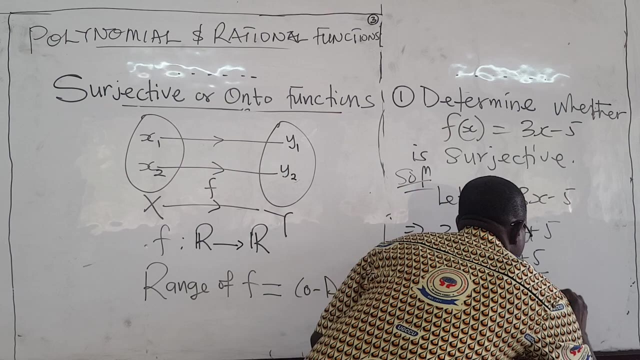 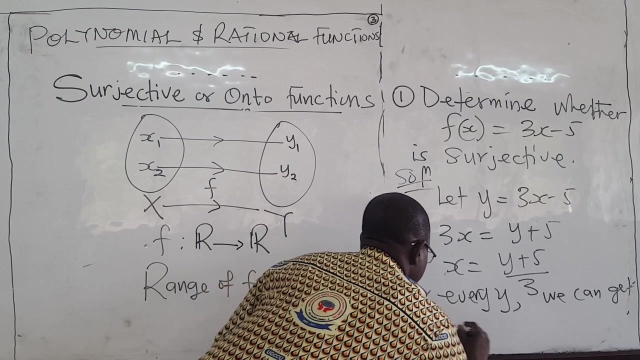 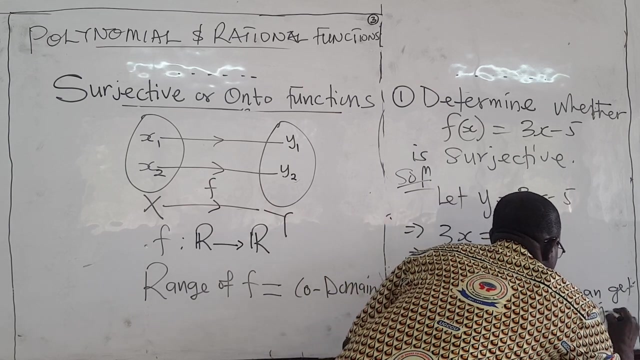 number, a negative number, a zero, whichever y I pick, as long as it's real, I can get a corresponding value of x. Okay, So for every, for every, every y we can, we can get, I see, and it has. hence f is subjective. Okay, So after you do this, you ask the question. 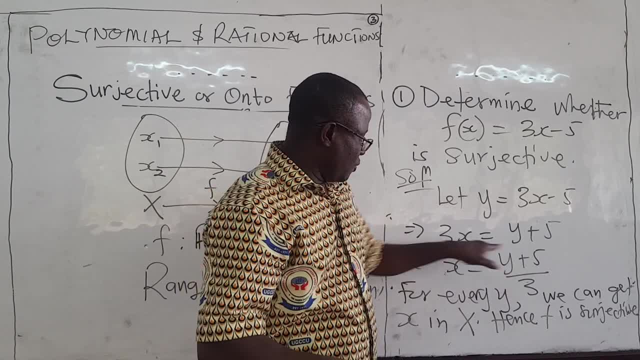 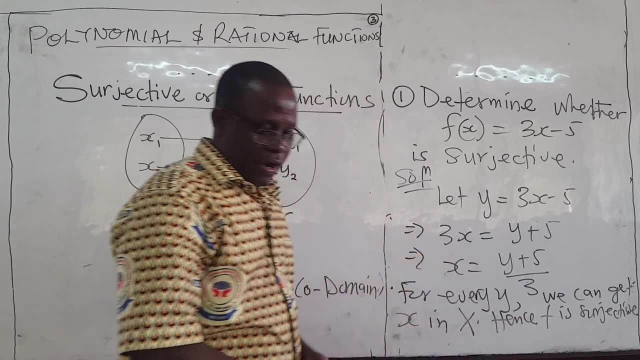 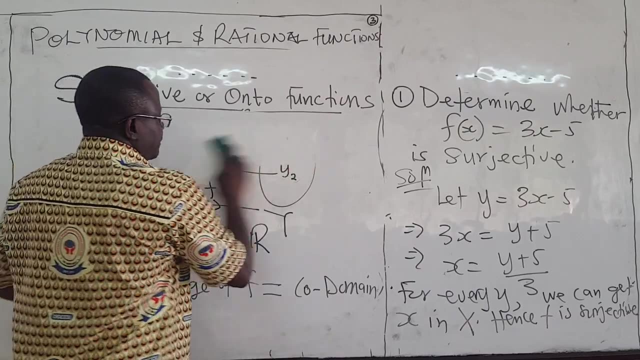 for every y that I pick, every y, will I get a corresponding x, And it's true. Okay, And so, once that is true, you conclude that the function is um subjective or onto. Okay, Um, let's do that. Well, you could, you could, you could also. 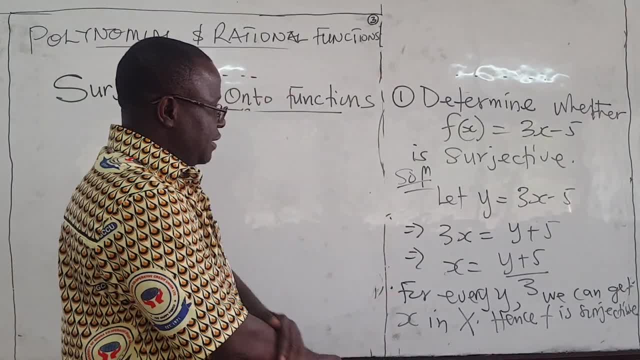 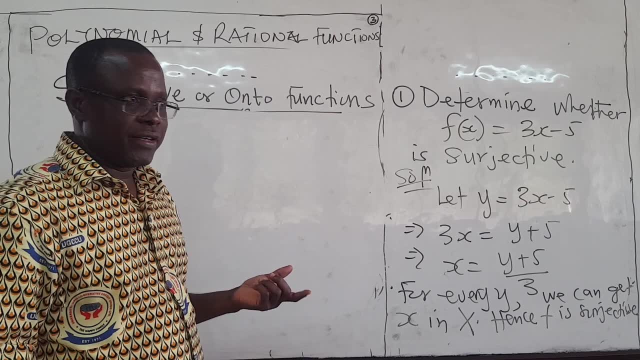 do do this. um alternatively, right, Um, use a, a second method. You could also try to uh to prove that the the rate is equal to the codomain right. So, if you like, before. 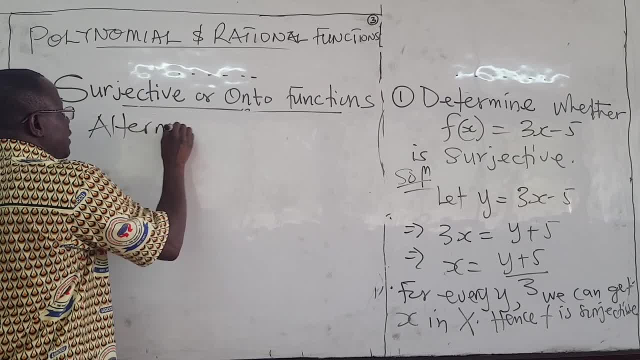 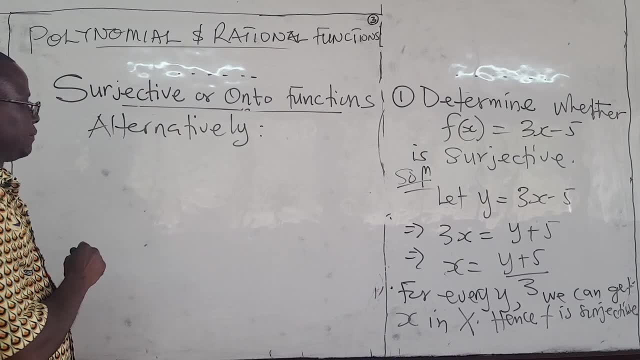 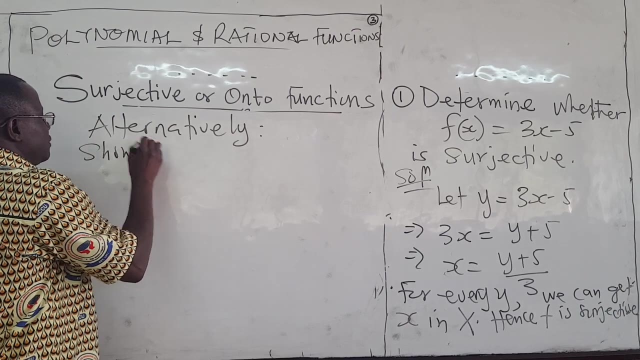 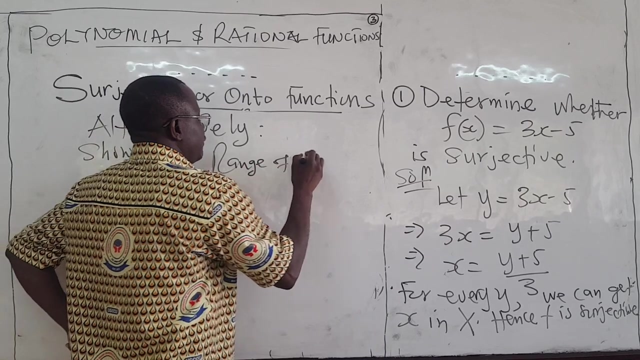 you do a second example, an alternative way of doing this. alternatively, right, You could say: um, can we show? try, okay. alternative way is to show, show that, show that, uh, range, range of f is the same as its codomain. All right, This is an alternative. way of showing that it is subjective. Okay, So now. so I, I I just find out that the this is the codomain, So I I think you can see, you can? you can see what I'm showing. here. okay, It's the codomain. So, um, I want to now, I want to first, I want to, I want to first, I want to explain how I can um work with this, this codomain, because 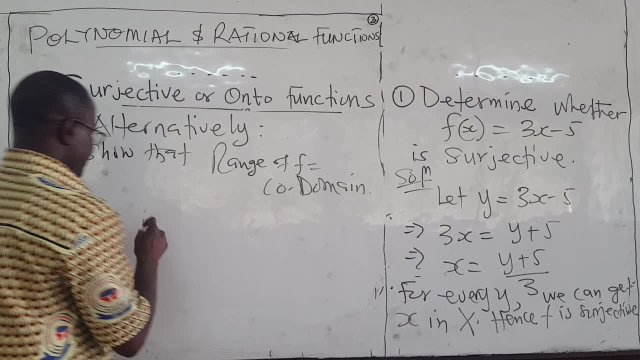 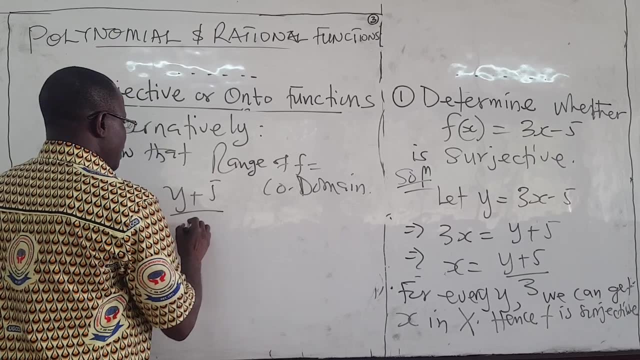 you can see that it is subjective. Okay, So now, um, I'm going to work with this code. We got here right. So if you were solving, you go to the same step. x is equal to y plus 5 over 3.. 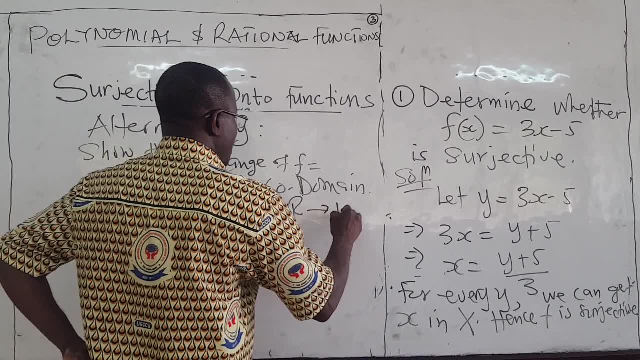 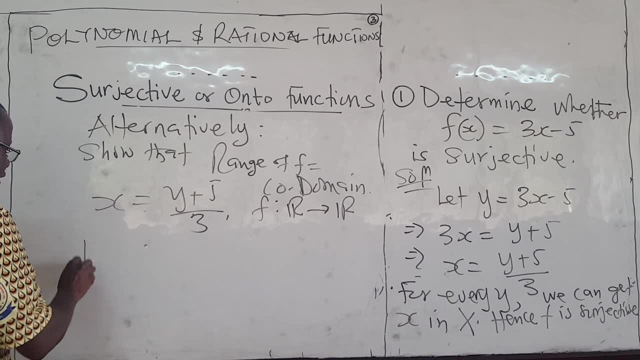 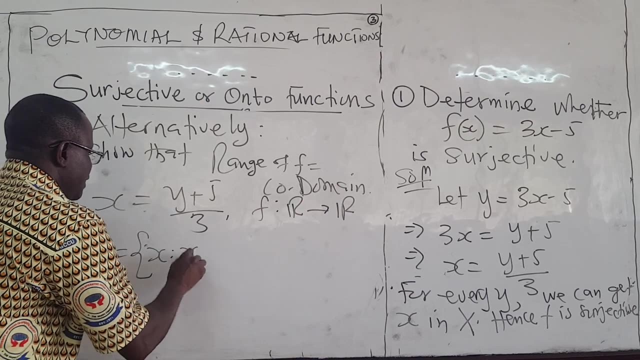 Remember, f is from r to r, a set of real numbers to real numbers. So we get there. and what is the domain? You see that the domain- let me shorten it, domain of f is x of. sorry, not the domain. we want the range, okay. 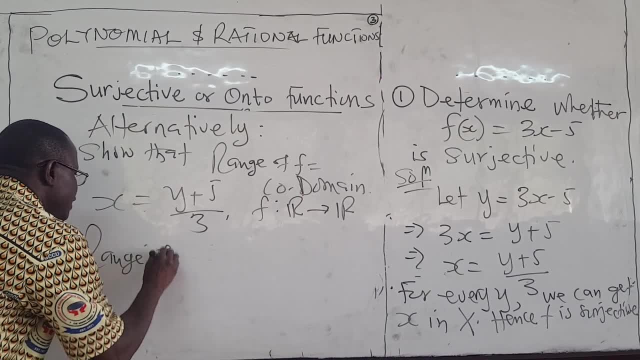 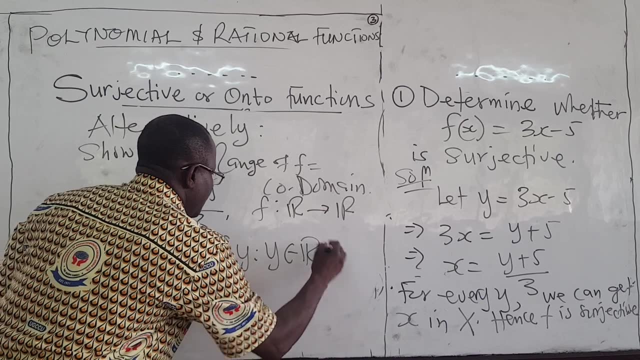 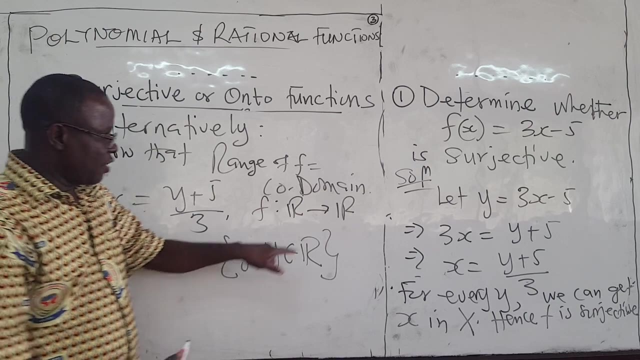 So range, range of f is all y, such that any real will do right, Any real number. So the range is a set of all real numbers. Okay, All right, And the co-domain is also the set of all real numbers. 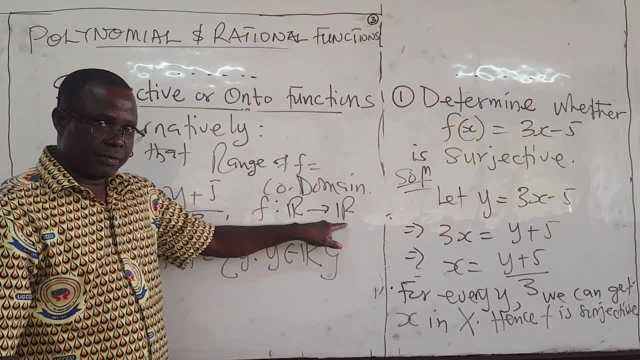 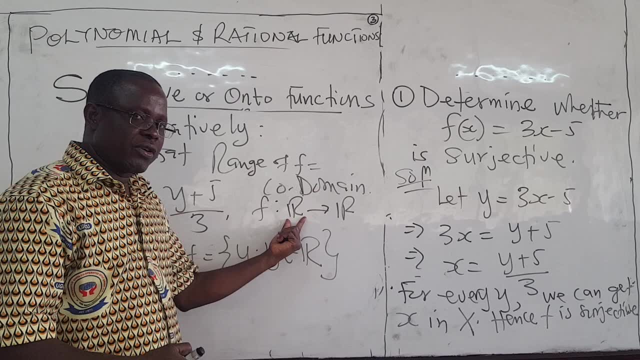 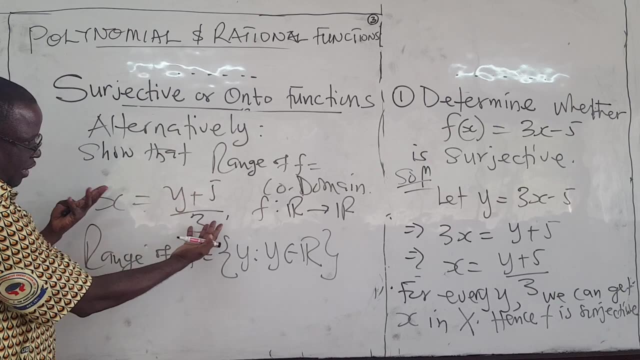 So the range is equal to the co-domain. All right, Remember, I said that when you're doing the function, you assume that it's taking elements from real to real. Okay, So the co-domain is a set of real numbers. So we have shown that from here. after you do this, we have shown that from here, the range is a set of all real numbers. 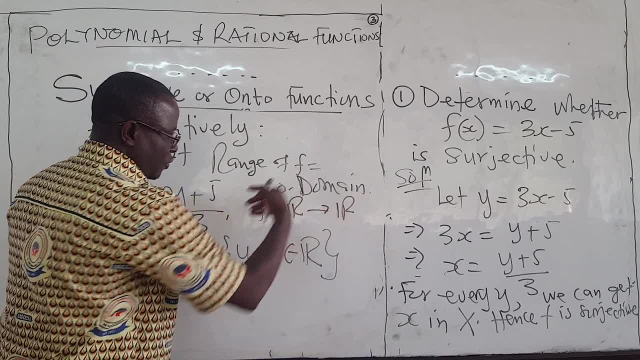 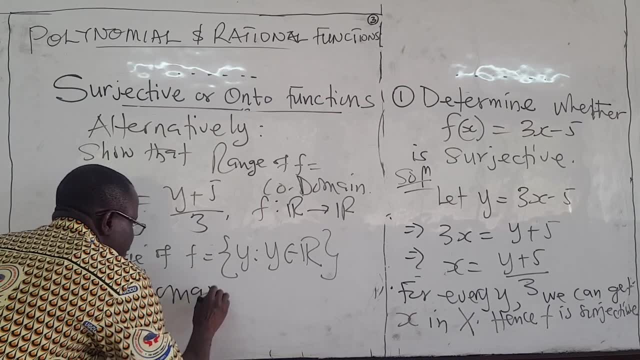 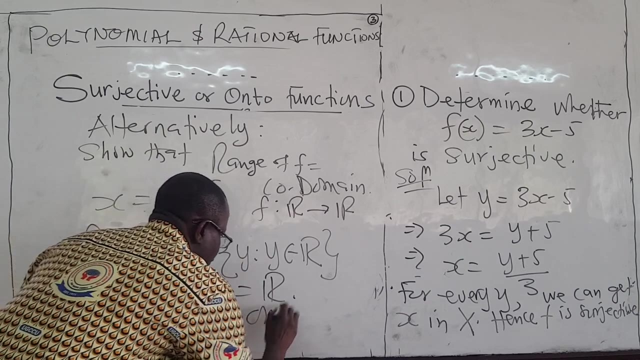 and a set of all real numbers. It's the same as the set in the co-domain. Therefore, and the co-domain- let's just do this co-domain- is also the set of real numbers. Hence f is onto outside the t. 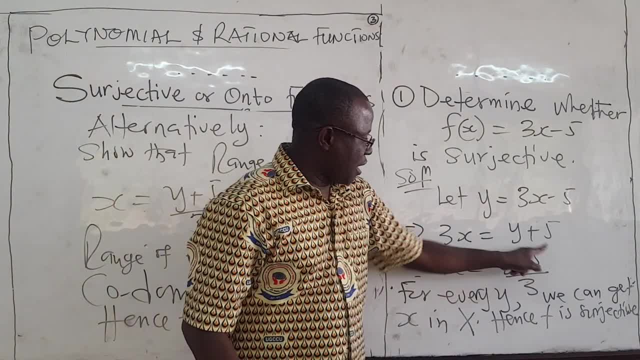 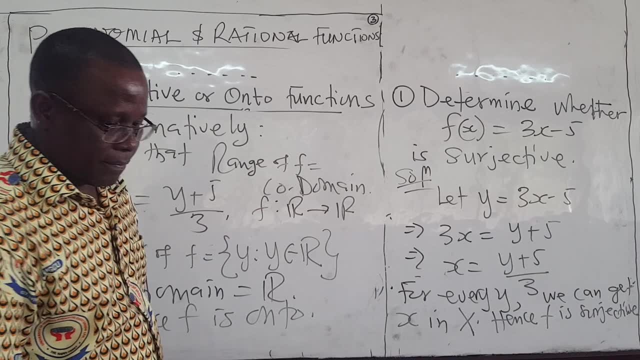 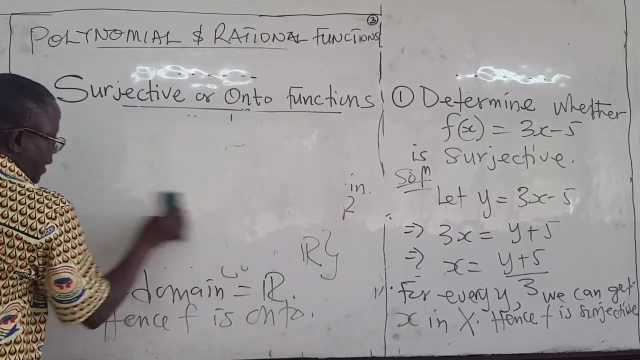 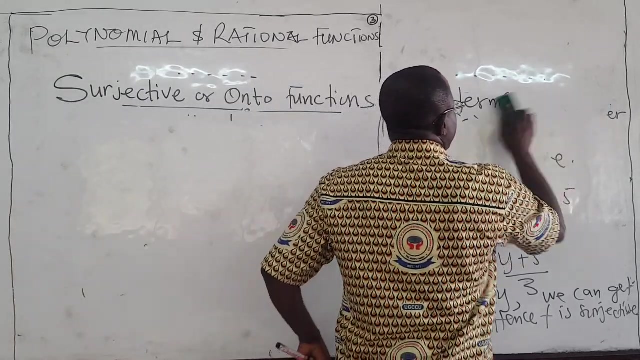 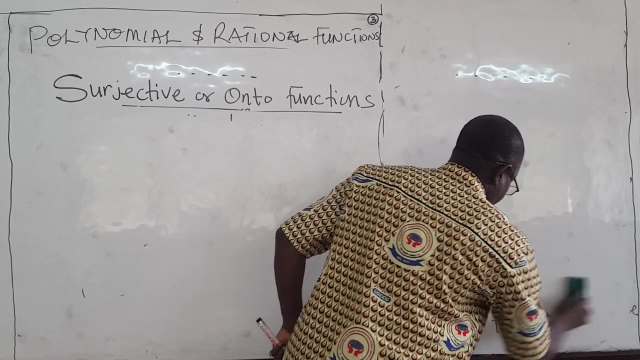 Okay, Whichever way, you still have to arrive at this expression here and make a conclusion. Good, So let's do a second example. Let's do a second example. So let's take a different function. So let's take f of x is equal to. let's do 2x squared, probably. 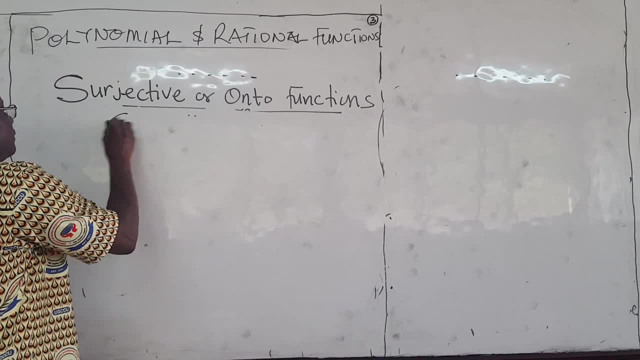 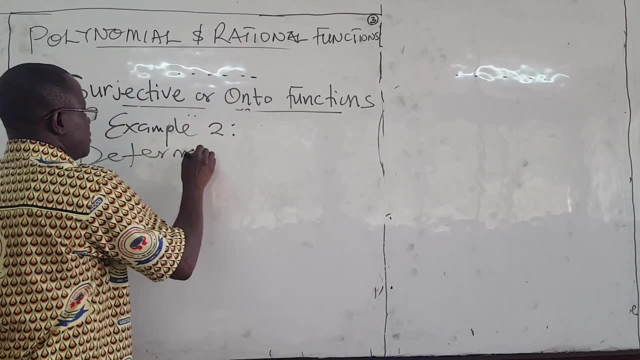 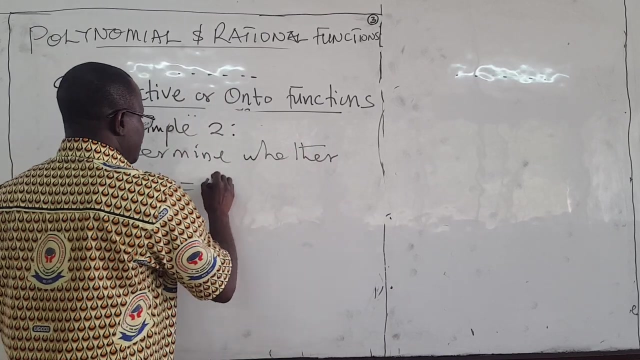 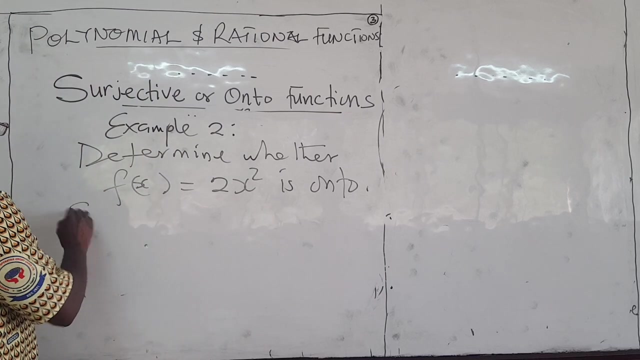 So let's try Example 2.. Example 2. Determine whether f of x is equal to. let's do the simple one: f squared is onto or subjected. Okay, Same thing, We're just going to use the same approach. 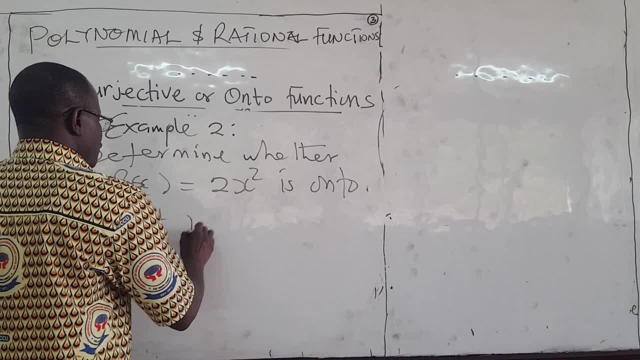 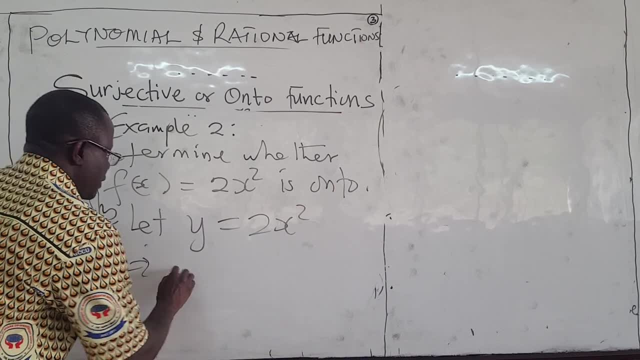 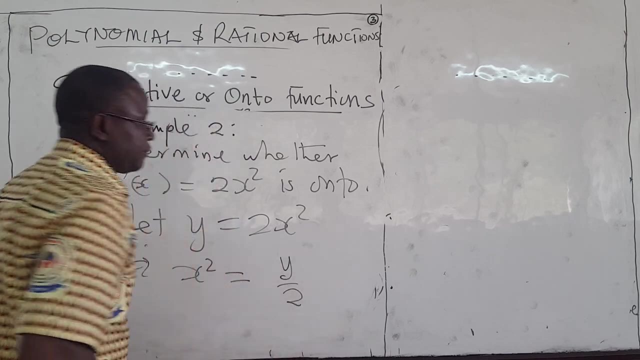 Let's assume you are finding the array right. So let y equal to 2x squared. I'm solving for x, so I divide x by 2.. So x squared is equal to y over 2, right, Okay, Let's go here. 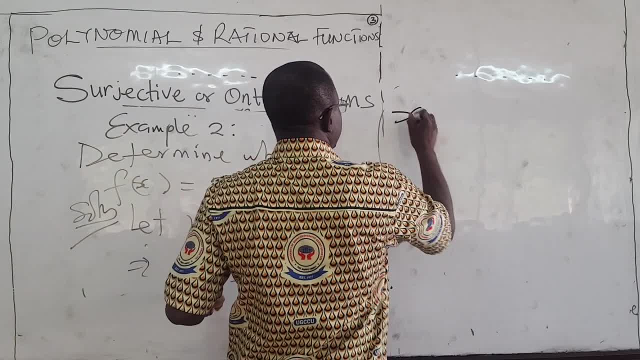 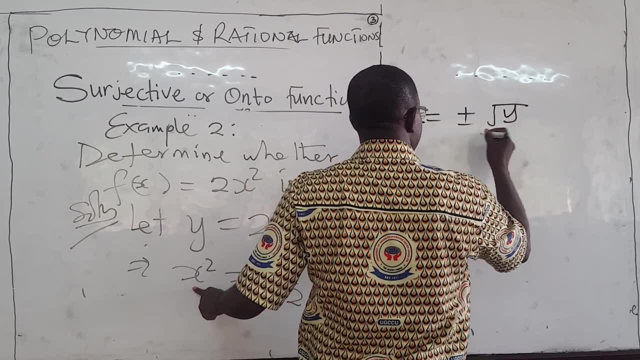 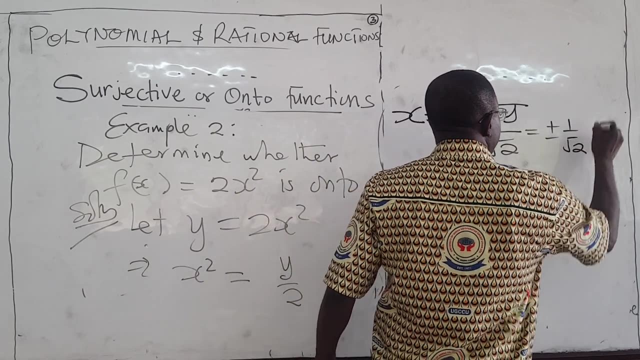 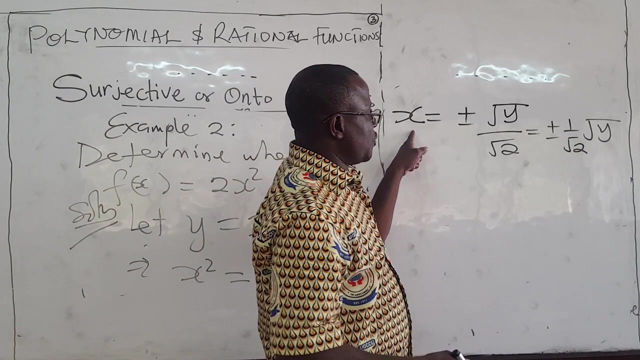 Which means x is plus or minus. So x is equal to plus or minus square root of 1.. y over square root of 2.. I'm going to write it in a nicer way. Okay, Maybe I should use 4.. But that's fine. 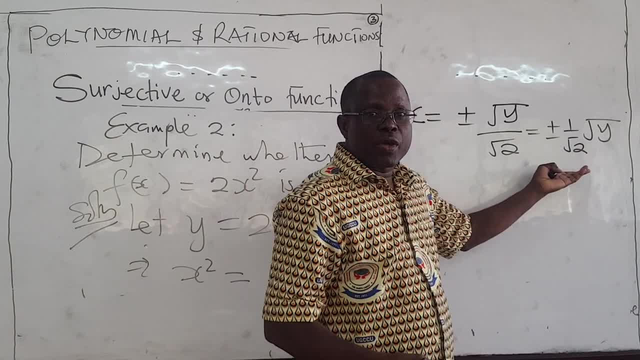 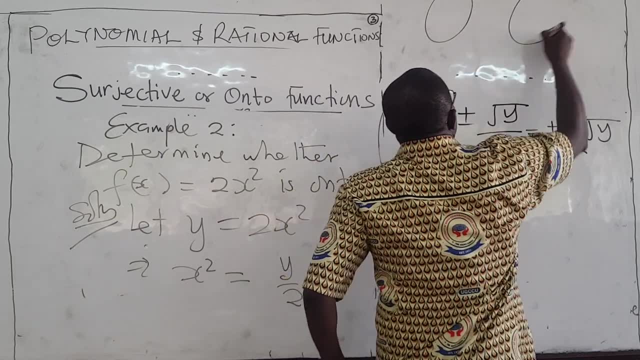 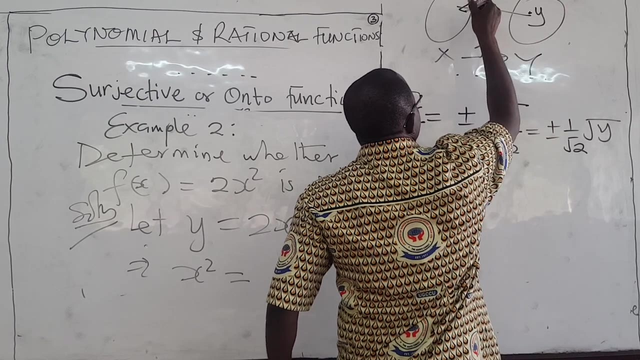 So x is equal to this. It's a number. So once you are here, you ask the question. All right, Remember, If I pick any y, if I pick any y from here, I might get a corresponding x here. All right, 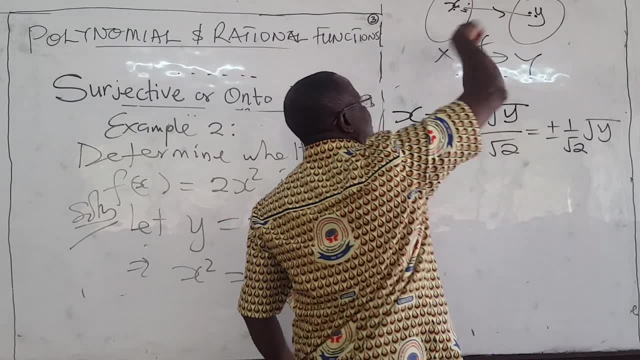 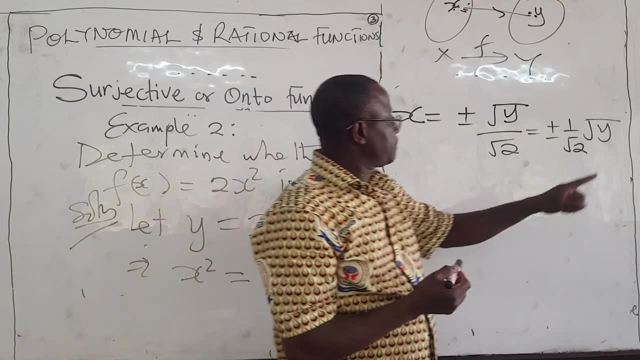 This is going here. So for every y it has to be x, For which f of x is y. All right, For all real numbers. Now you notice that if we pick a negative number, if y is less than 0,, 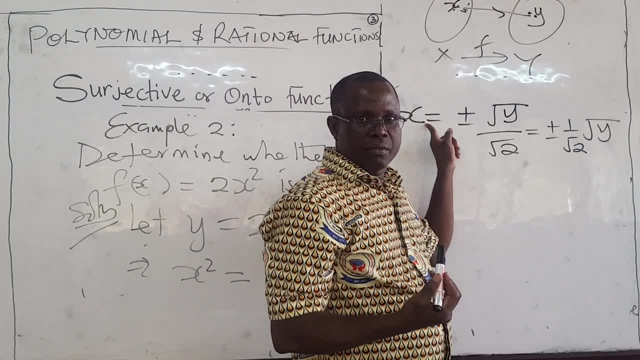 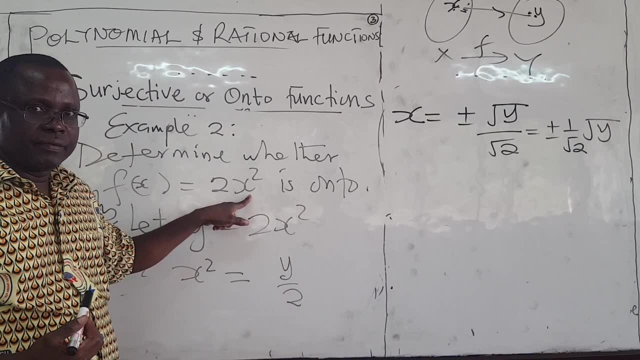 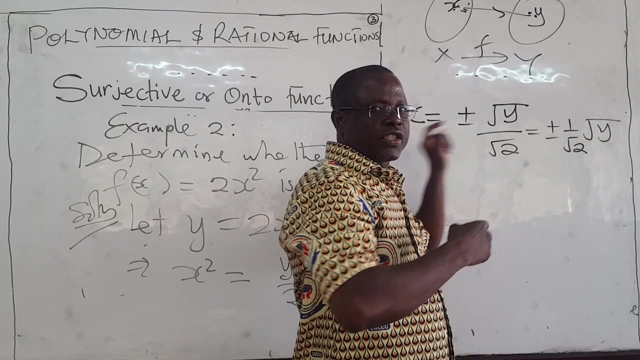 we can't get any real x. You see that, And so, for that matter, the function 2x squared is not suggestive. It is not because you can't pick any y, any real number, and get a corresponding x. Right. 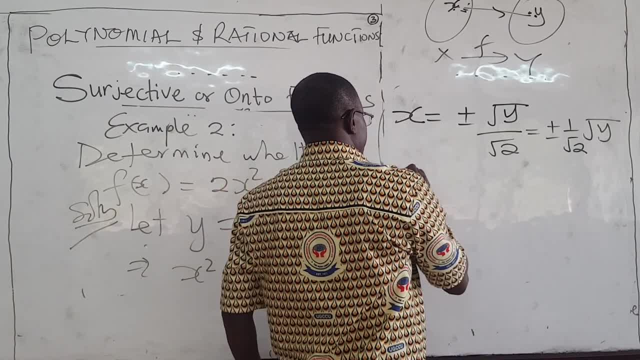 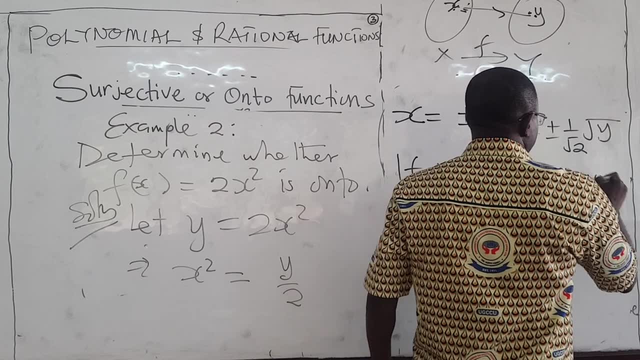 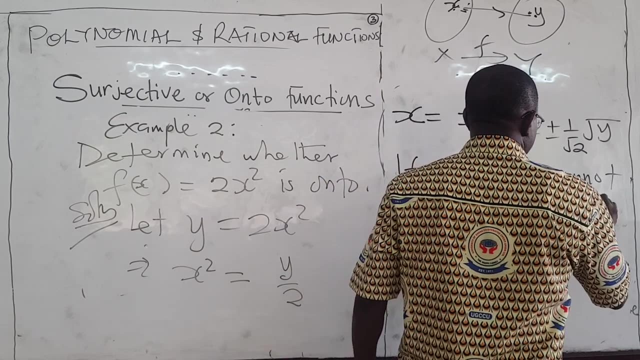 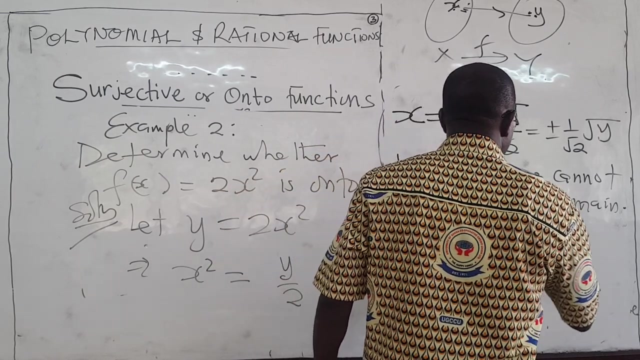 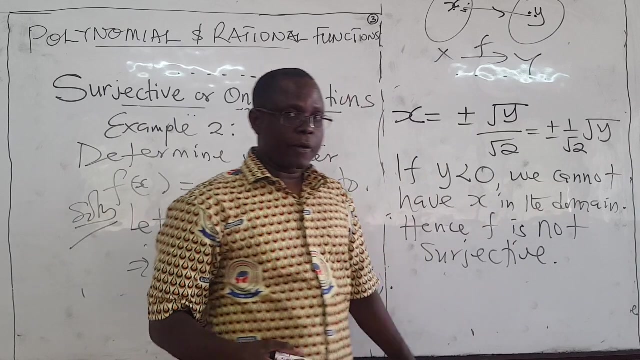 In its domain. So if y is less than 0, you cannot, you cannot have, you cannot have x in the domain, Okay, And f is not suggestive, Okay. So really, that is the basic idea. You want to show that, after you've done this,